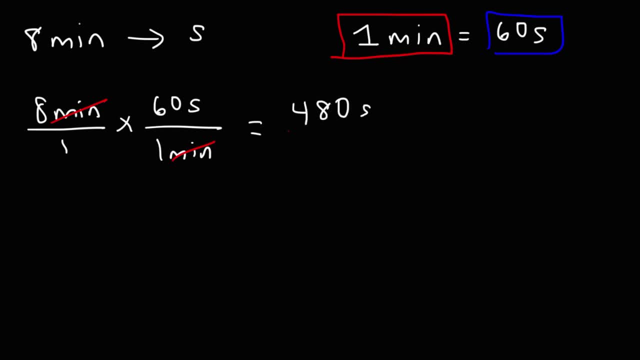 this will be 480. And that is the answer. So 8 minutes is equal to 480 seconds. So now it's your turn. Go ahead and convert 5 minutes into seconds and 7.2 minutes into seconds. So for the first one, 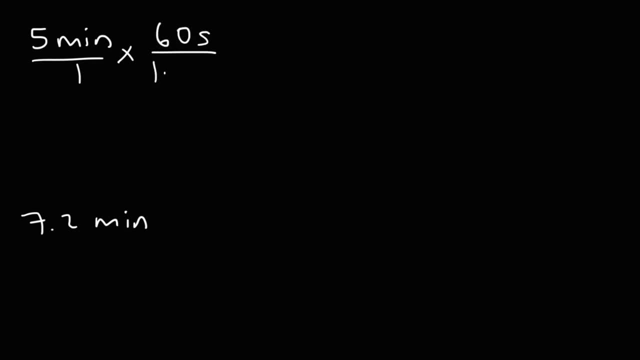 we're going to multiply it by 60 seconds over 1 minute so that the unit minutes will cancel. So it's 5 times 60.. 5 times 6 is 30.. Add the 0. That gives us 300 seconds. 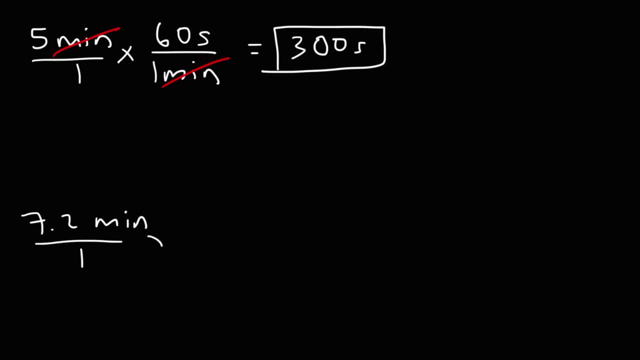 Now for the one on the bottom. we're going to do the same thing. We're going to multiply it by 60. So this is 7.2 times 60. And let's use a calculator for that. So this is going to be equal to 432 seconds. 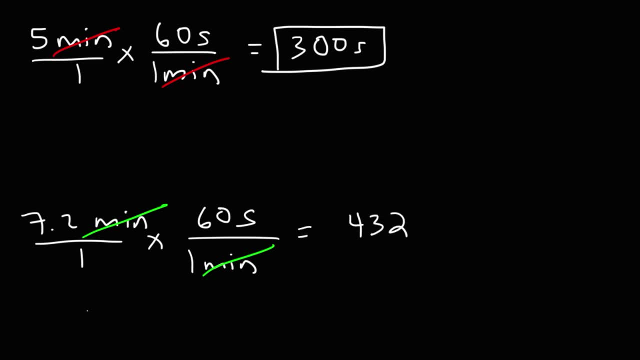 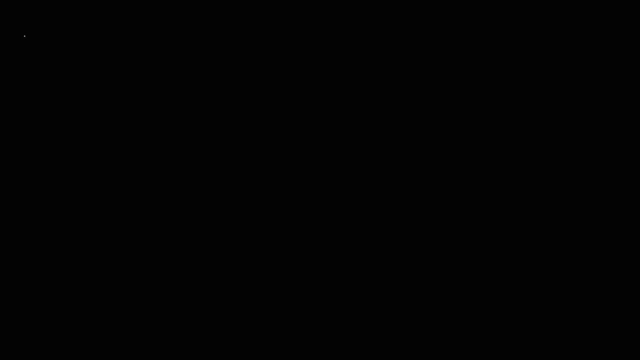 So now you know how to convert from minutes to seconds. Now let's say: if you are given 6 minutes. Now let's say, if you are given 6 minutes and 15 seconds, how do you convert that to seconds? Go ahead and try that. 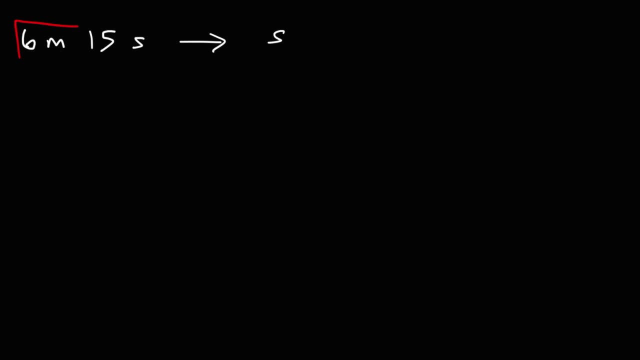 Now what you want to do first is you want to convert the 6 minutes portion into seconds. into seconds, we know that there's 60 seconds in one minute, And so it's going to be 6 times 6,, which is 36.. 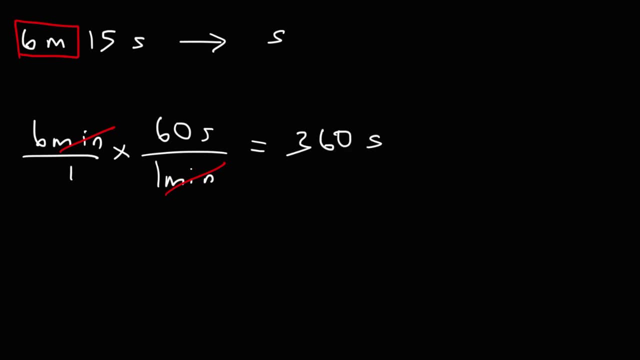 Add the 0, you get 360 seconds. So 6 minutes is equal to 360 seconds. To find 6 minutes and 15 seconds, all we need to do is add an additional 15 seconds. So this is going to give us 375 seconds. 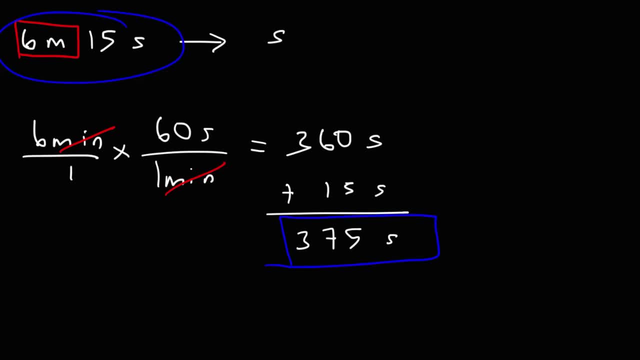 So that's how we can convert from minutes and seconds into seconds. So, for the sake of practice, go ahead and try these problems. Let's say you have 7 minutes 35 seconds and 9 minutes 42 seconds. Go ahead and convert both of those quantities into seconds. 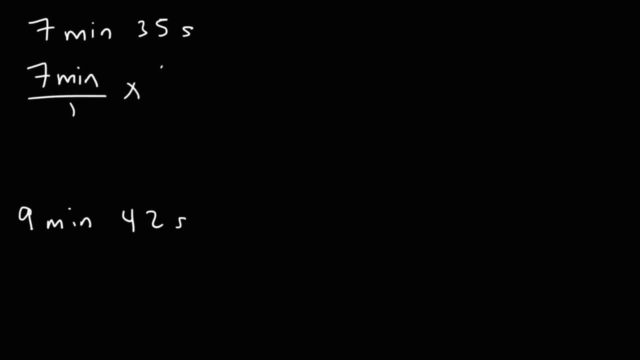 So let's begin by starting with 7 minutes and let's convert that into seconds, So the unit minutes will cancel. 7 times 6 is 42, but if you add the 0, you get 420.. So 7 times 60 is 420. 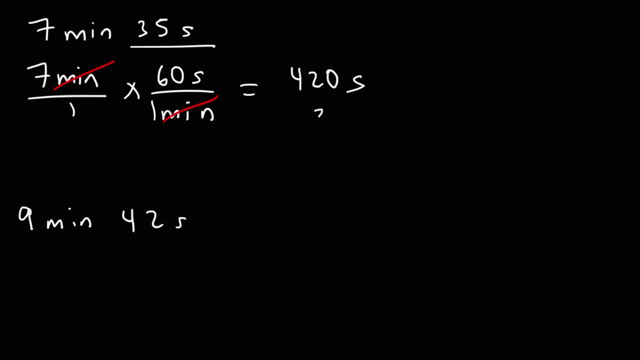 So we have 420 seconds, and now let's add 35 to it. So 5 and 0 is 5, 2 and 3 is 5.. This gives us 455 seconds. So, as you can see, these problems are not too difficult. 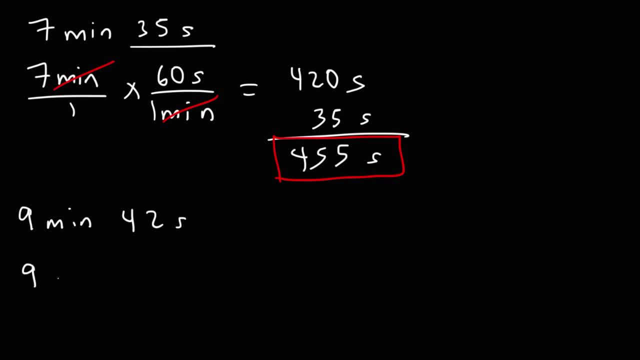 They're doable. Now let's try the next one. So we have 9 minutes. We're going to multiply it by 60 seconds per minute. So what's 9 times 60?? We know, 9 times 6 is 54.. 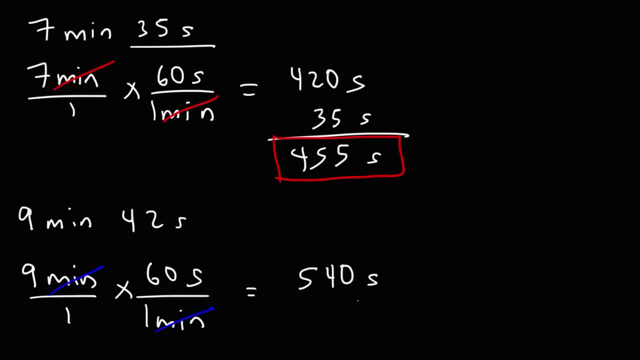 Adding a 0, that tells us that 9 times 60 is 540. And then let's add 42 seconds to it, So this is going to give us 540. And this is going to give us 582 seconds. So that is the answer. 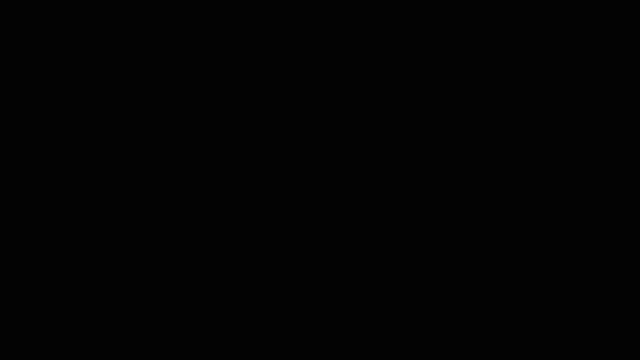 Now let's talk about how to go backwards, How to go from seconds to minutes. So let's say, if we have 180 seconds, How can we convert that into minutes? Now, going from minutes to seconds, we needed to multiply by 60.. 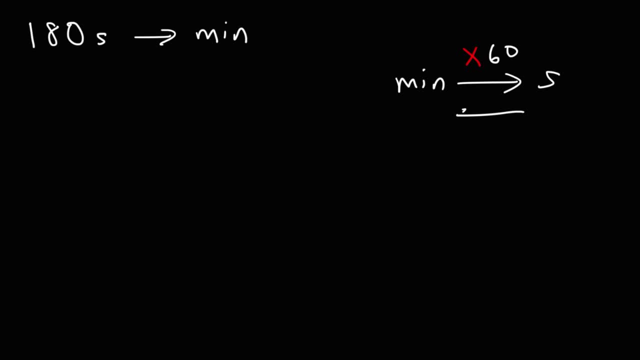 60, because there's 60 seconds in a minute. Going backwards from seconds to minutes. what we need to do is divide by 60.. So for this example, we know our conversion factor is this: One minute is equal to 60 seconds. 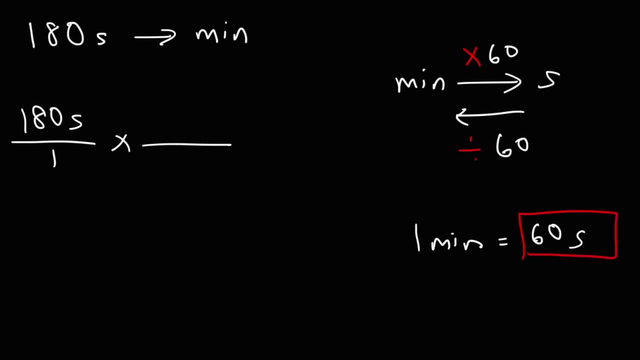 Now, where should you place the 60,? excuse me, where should you place the 60 seconds? On a top or on a bottom? Notice that the unit seconds is 60 seconds. The unit seconds is on the top left, So we want to put the unit seconds on the bottom right. 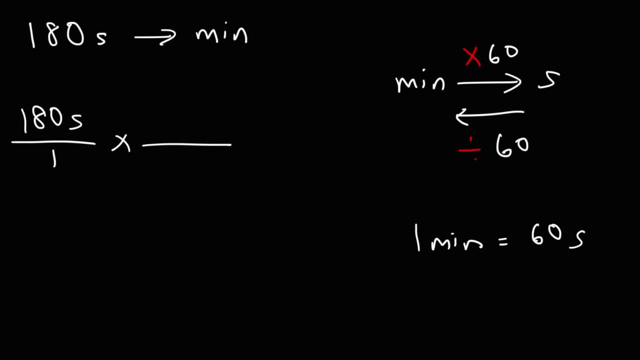 so that they cancel, leaving us with the unit minutes. So we're going to put 60 seconds on the bottom, one minute on the top, So the unit seconds will cancel. And now we need to divide. So it's 180 divided by 60.. 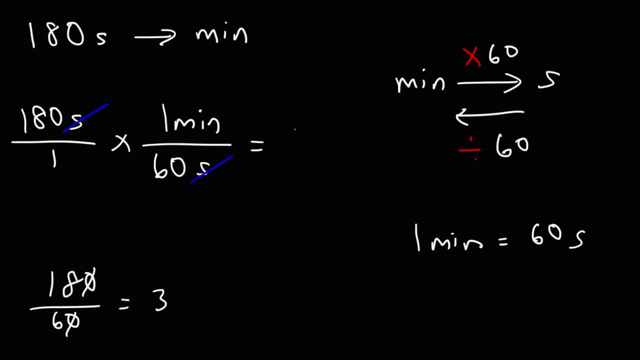 We can cancel the zero and it becomes 18 divided by six, which is three. So 180 seconds is 180 seconds divided by 60.. So 180 seconds is 180 seconds divided by 60.. So 180 seconds is 180 seconds divided by 60.. 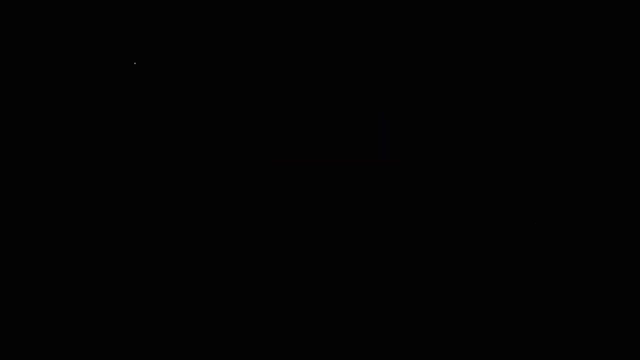 So it's 180 seconds. So it's 180 seconds equal to three minutes. Here's two other examples that you can try. Go ahead and convert 460 seconds into minutes. Go ahead and convert 460 seconds into minutes and then convert 800 seconds into minutes. 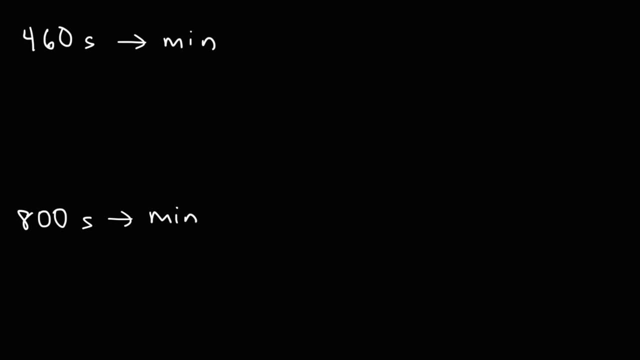 and then convert 800 seconds into minutes. So with the first one we're going to put 60 seconds on the bottom. as we said before, we want these units to cancel. we're going to put one minute on the top, so it's going to be 460 divided by 60 and that is 7.6 repeated. so you 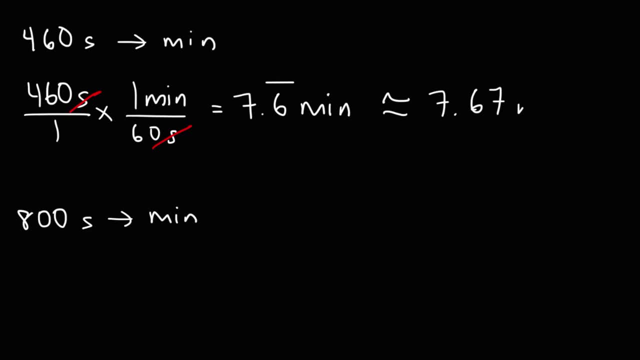 can round and say that's about seven point six, seven minutes. now let's do the same for the second example. we have 800 seconds and we're going to multiply by one minute divided by 60 seconds, so the unit seconds will cancel and it's just. 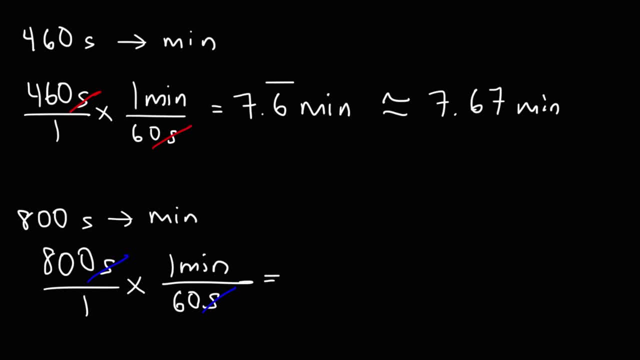 going to be 800 divided by 60, and so that's going to be 13.3 repeated, and so that's how you can convert from seconds to minutes now, earlier in this video we said that seven minutes and 35 seconds corresponded to four hundred and fifty. 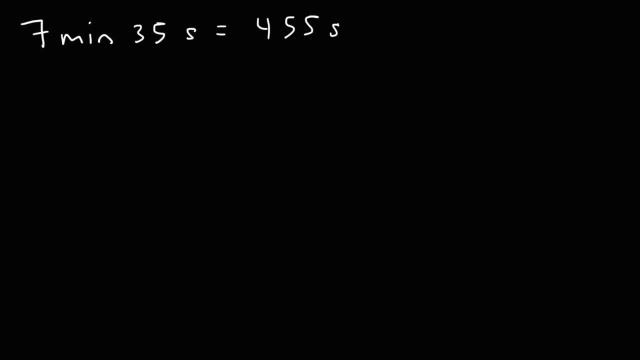 seconds. I mean 455 seconds. now here's a question for you: how can we convert back from 455 seconds to the result that we see on the left? how can we do that? what would you say? so here are the steps that you need to take, starting with 455 divided by 60. 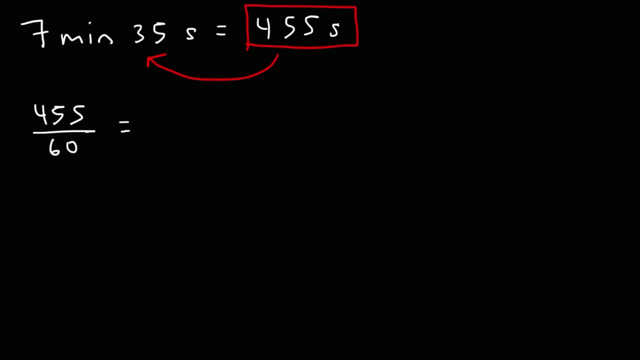 so this is 7.583 repeated. now the whole number portion, that is the seven. that's going to go with the minutes portion. what's left over? the .583 repeating? I'm going to add a few threes. take that and multiply it by 60. 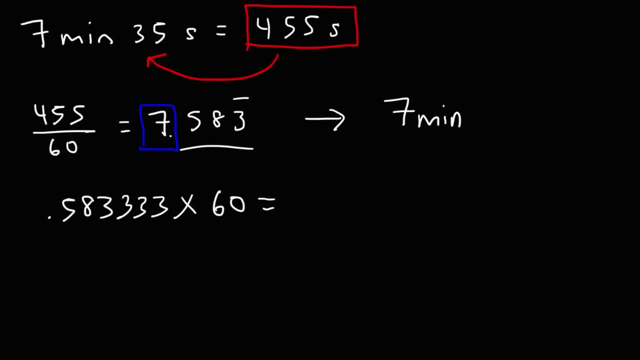 in this case you get thirty four point nine, nine, nine, nine, eight, which, if the threes goes on forever, this is going to be 35, and then you combine these two, so the answer is seven minutes and 35 seconds, if you want to check your answer. 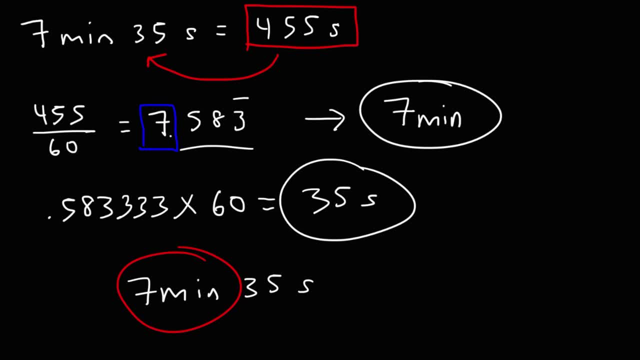 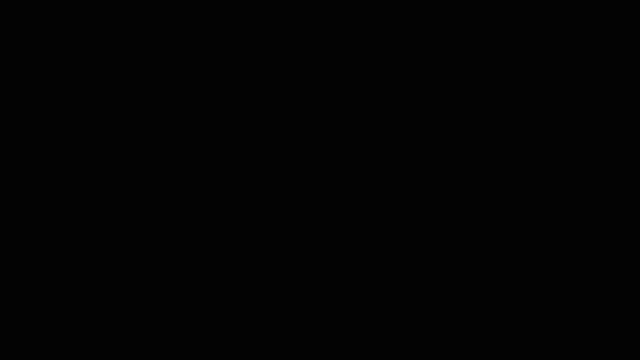 take seven multiplied by 60, that will give you 420. add 35 to it, that will give you 455. so that's how you can convert from seconds to minutes and seconds. so I'm going to give you some more examples. let's say, if you have 835, 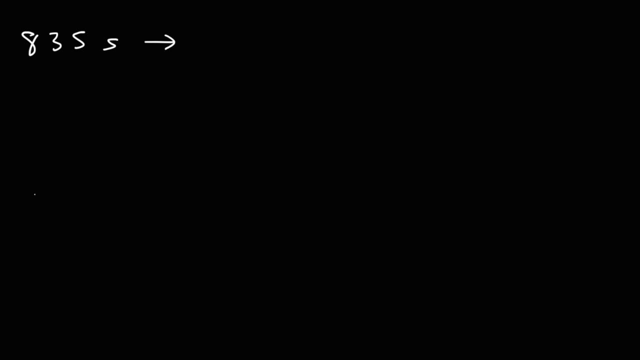 seconds, convert that to minutes and seconds. and if you have, let's say, five hundred and sixty-eight seconds, convert that to minutes and seconds as well. so, starting with the first one, 835, we're going to divide it by 60, and so that's going to be thirteen point nine, one, six, repeating. so we're going to take the 13.